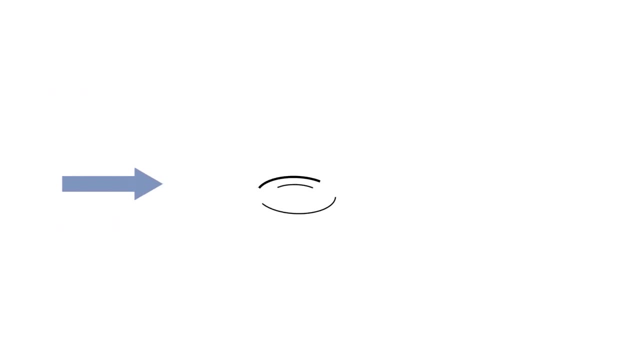 it misses the point for engineering students. Instead, we can show engineering students how to work with engineering tools while learning physiology concepts, Introducing a student to concepts such as systolic and diastolic blood pressure and QRX complexes, while, at the same time, introducing them to signal conditioning. 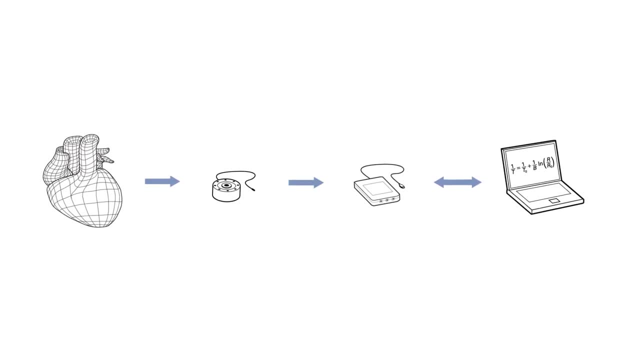 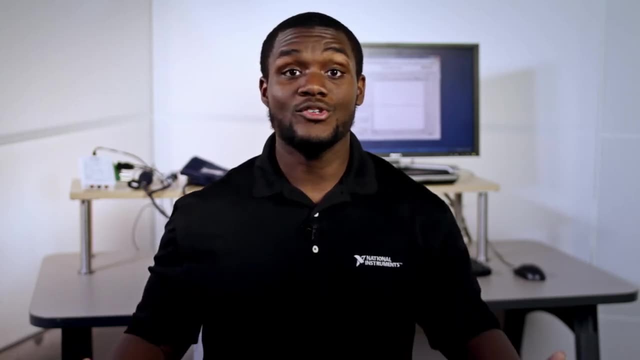 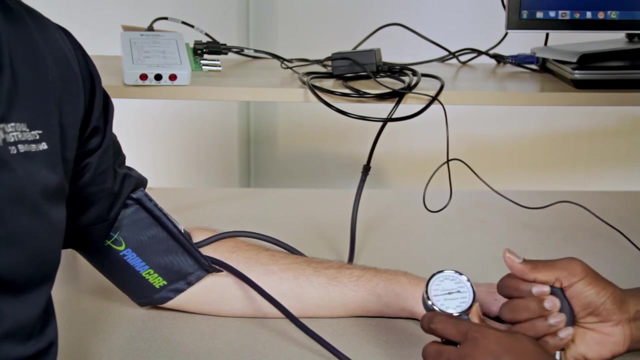 and an analysis concepts is a more effective way for them to learn about physiology because it's in a relevant context such as engineering. So I'm going to walk through a specific example of teaching students about exercise physiology using an engineering system. We'll measure heart rate and blood pressure of a subject at rest and then during exercise and 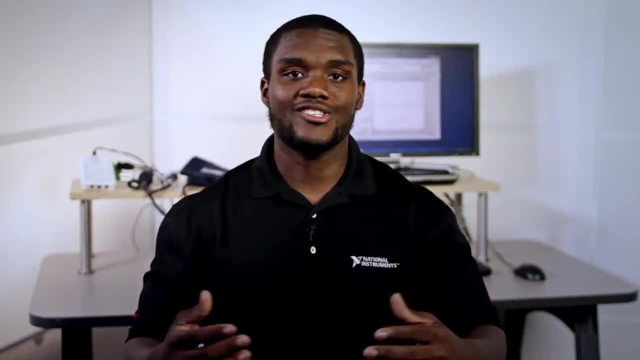 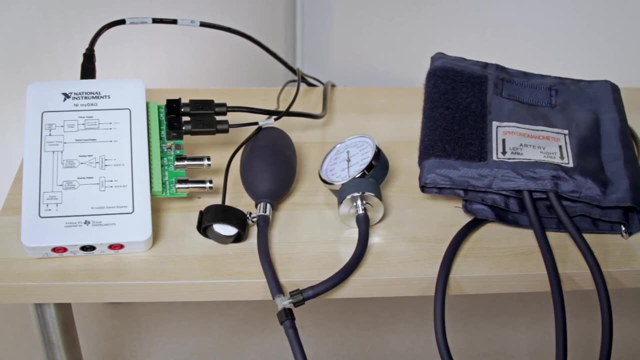 compare these values to their calculated target heart rate. So let's get started. An important part of this process is the engineering student actually understanding what the system is doing and its parts. So here I have a blood pressure cuff hooked up to a pressure sensor, a pulse sensor. 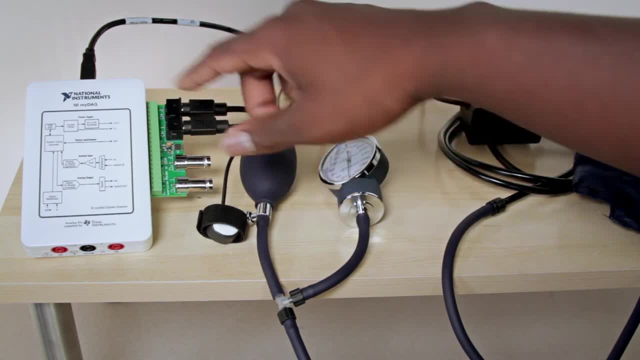 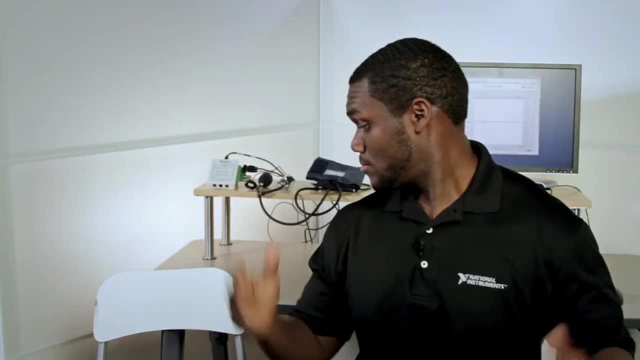 and both of these signals are being run into my measurement system. In this case, we're using a MIDAC. To start my experiment, I'm going to need a test subject Now. what we have to do is hook the blood pressure cuff up to his arm and the pulse sensor to his 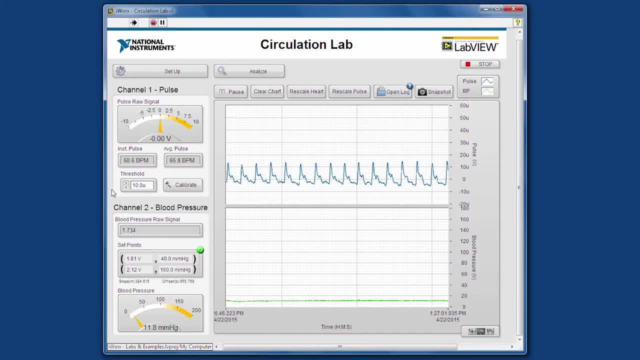 finger and we can start taking some data. So the two signals that we're acquiring are going into our virtual instrument written in the lab lab view. Now we can see that our test subject still has a pulse. Now, if I increase the 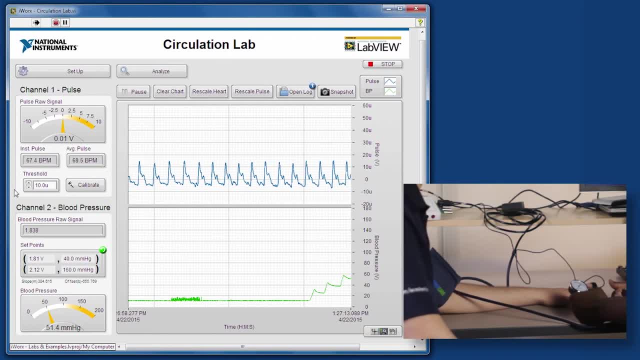 pressure in the cuff, we'll slowly start seeing our pulse disappear. At the moment that our pulse disappears, we can call that the systolic pressure. Now, if I slowly release the pressure in the cuff, the moment that we see our pulse reappear and stabilize, we 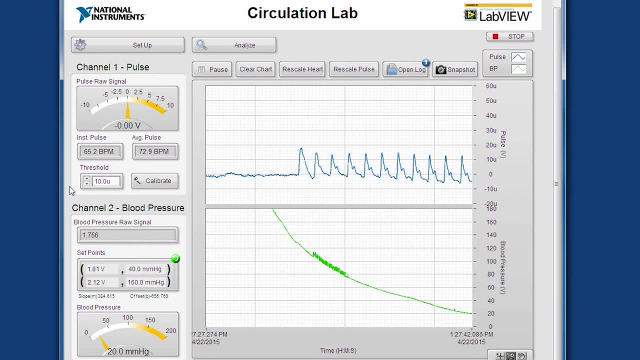 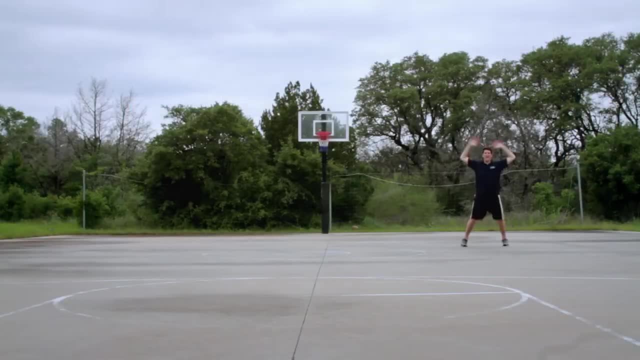 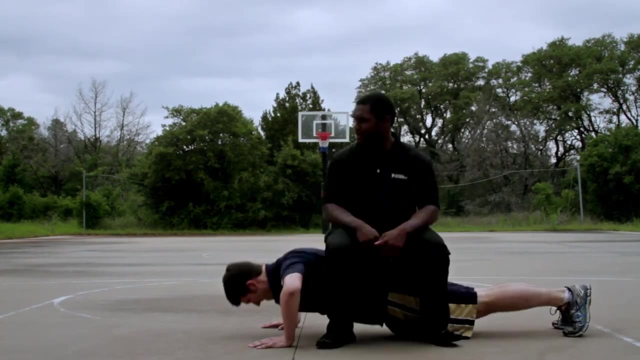 call that our mean arterial pressure, And with a little bit of math we can calculate our diastolic pressure. So now our test subject is going to go work out and then we're going to take the same measurements when he gets back. Now that he's back, we're going to go.